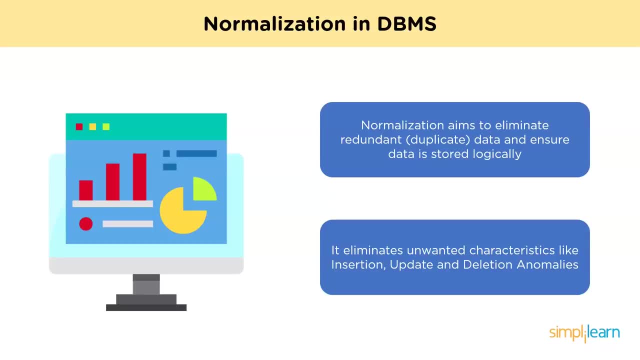 There can be the possibility of redundancy being present in the data, So normalization aims to eliminate this redundancy from the data and ensures data integrity. Using normalization techniques, you can split a large table into smaller tables and define relationships between them to enhance the clarity in organizing data. It also removes anomalies like insert, update and delete anomalies. 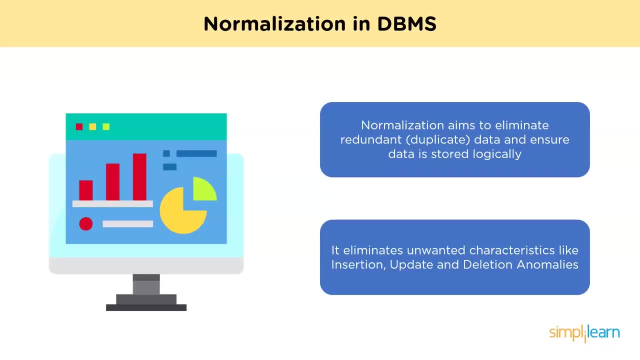 In insert anomaly. the values such as null are not allowed to be inserted in a column, So a record about an entity cannot be inserted into the table without first inserting information about another entity. So, for example, you cannot enter a customer without a sales order. 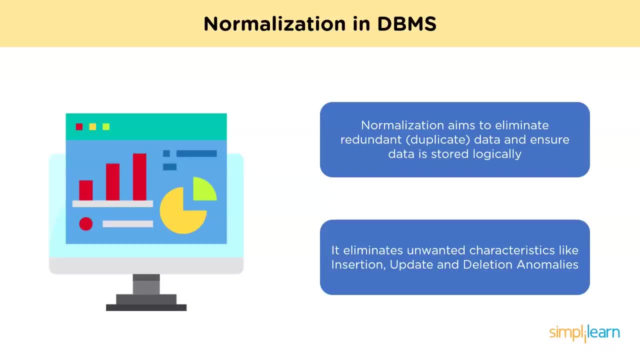 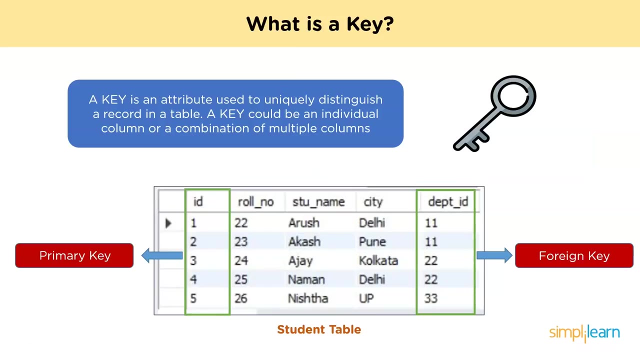 Now, in update anomaly, the data cannot be updated correctly because these same values occur multiple times in a column And in delete anomaly. the deletion of a record generates inconsistency as a result, as it gets deleted from more than one row. Now to understand how normalization works. 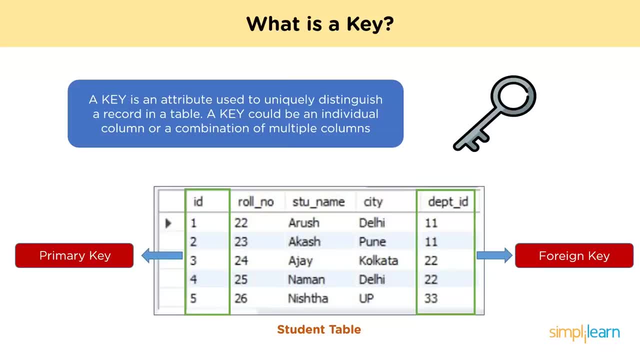 it is important to learn about keys in databases. A key is an attribute or a column that uniquely distinguishes or identifies a record in a table. A key could be an individual column or a combination of multiple columns. It is a very important part of relational database model. In reality, 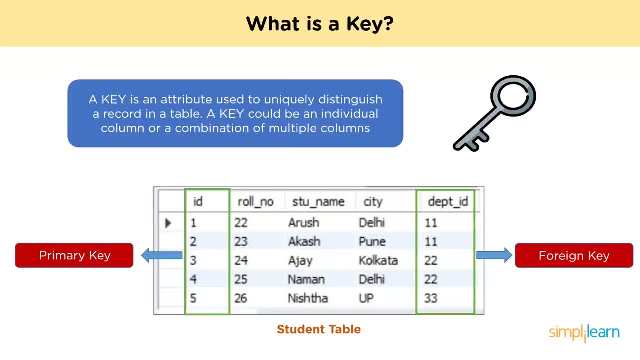 multiple tables are needed for storing the data and those tables are related to each other as well. To retrieve any specific record from a table, you need to apply some conditions. But what if there is duplicate data present and every time you try to fetch some data by applying certain conditions? 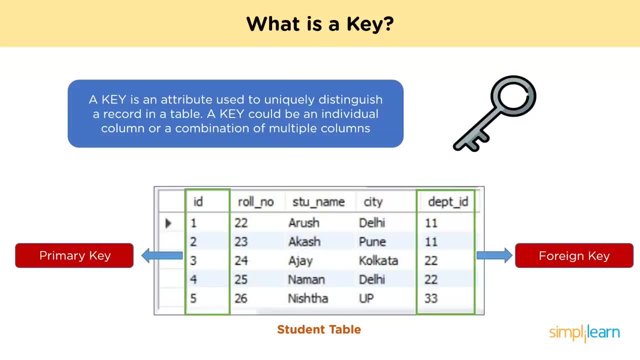 you get the incorrect result or the data. So to avoid these issues, we need keys in a table. Now, keys also help to establish relationships among the tables. So here you can see we have a student table and it has columns like the student ID. you have the student role number. 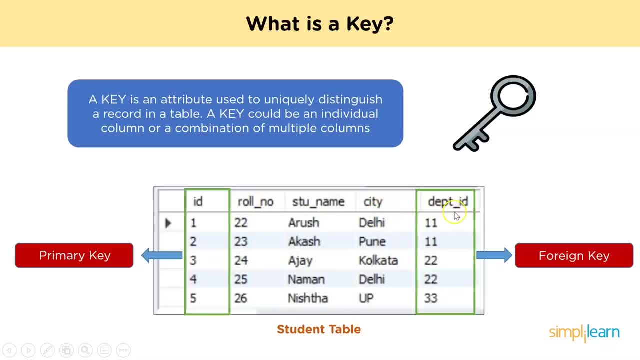 student name, the city to which the student belongs to, as well as the department to which the student belongs to. So in this table ID column is the primary key. You can also have the role number as the primary key, because this is the column from which you can identify individual. 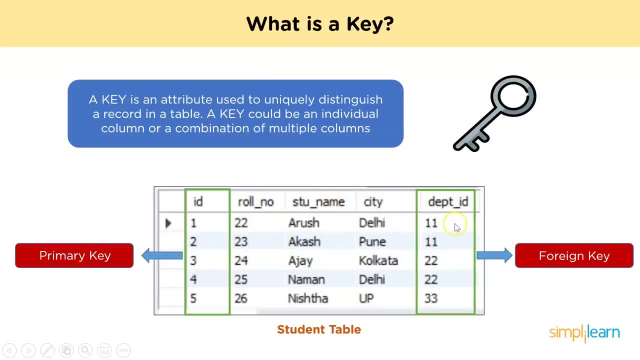 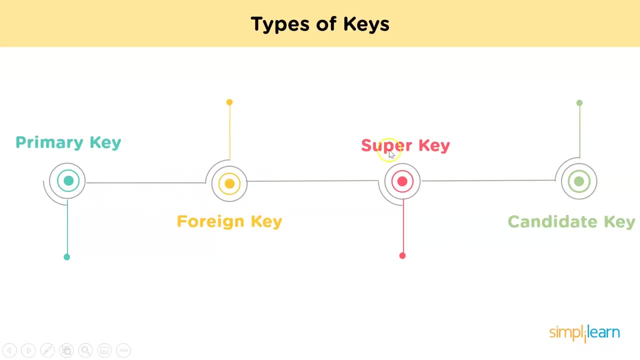 record for any of the students And here you can see department ID is called the foreign key. Just wait for a while. we'll learn about foreign keys in a while. Now let's look at the different types of keys in a database. So we have primary key, foreign key, super key and candidate key that we 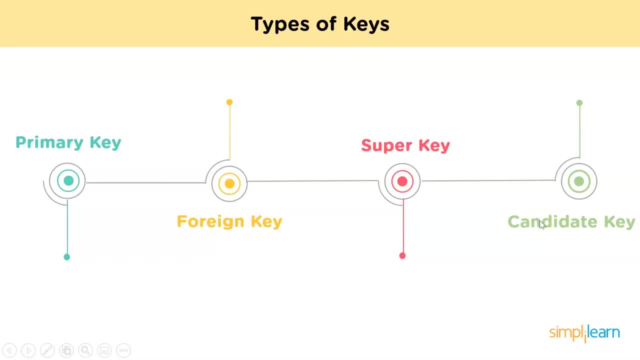 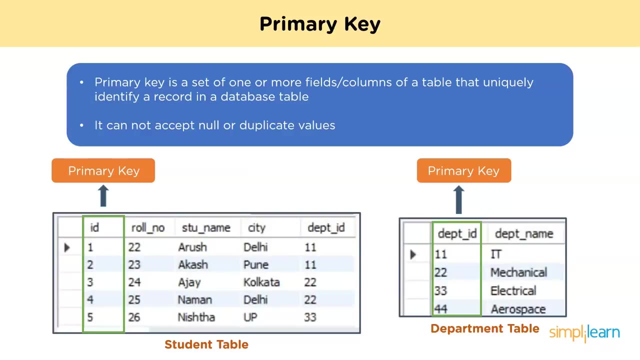 are going to discuss in this video. There are other keys as well, like the composite key, alternate keys, Cool, Now let's understand what is a primary key. So primary key is a set of one or more fields or columns of a table that uniquely identifies a record in a database table. It cannot accept null. 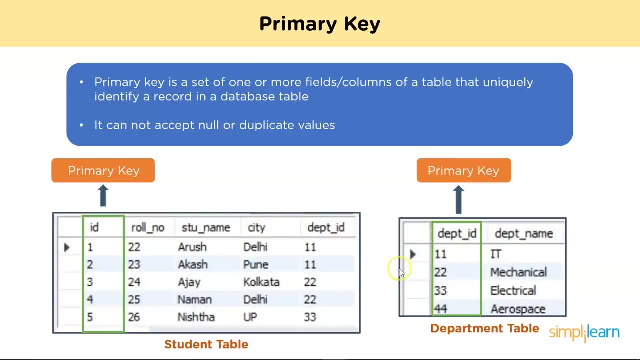 or duplicate values. Here you can see we have two tables. The first is the student table and the second one we have is the department table. So in the student table we have columns such as the student ID. we have the role number column, student name, city and the department ID to which the student belongs to. 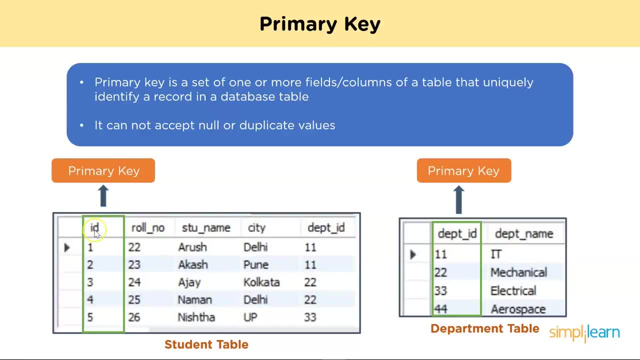 So in this case the primary key will be student ID, because you can see, all the values are unique and there are no repetitions, as in there are no duplicate values for the ID column. You can also consider the role number as the primary key, because in a 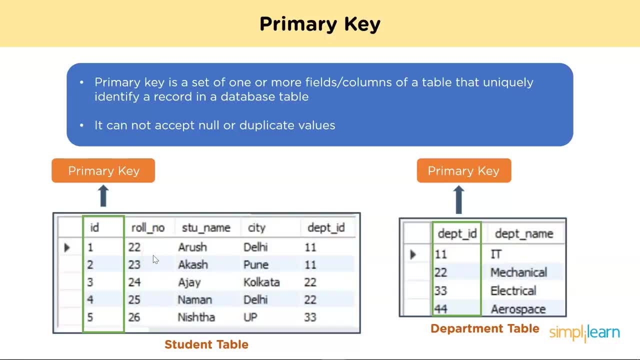 college or in a school, the role number for each student in a class would be unique. So here also you can see the role numbers are all unique, but you cannot have student name, city and department ID as the primary key, because there can be two students with the same name. 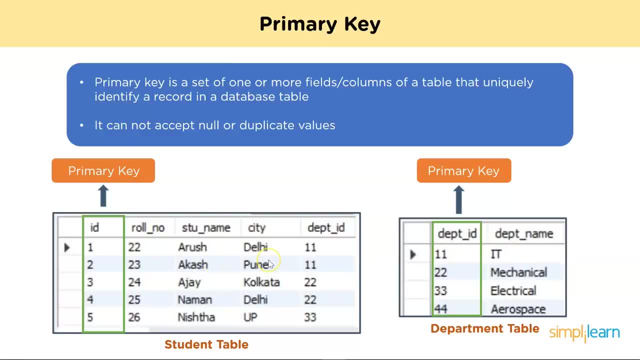 Similarly, there can be different students belonging to the same city and there could be a lot of students from the same department. So these three columns cannot be the primary key columns. Only ID and role number can be the primary key columns. Similarly for the department table. 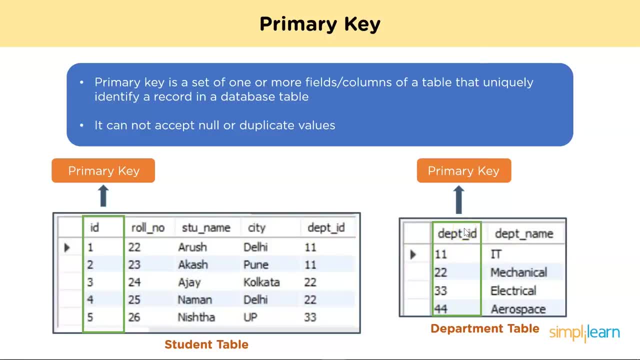 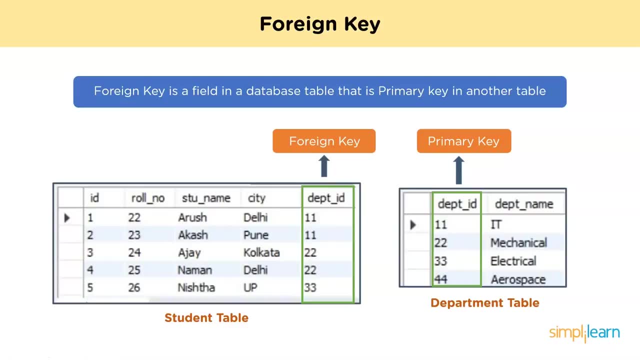 the department ID is the primary key. Now moving on. next we have foreign key. So foreign key is a table in a database that is the primary key in another table. So here we have the same tables as we saw in the previous slide. So here we have the student table and the department table. 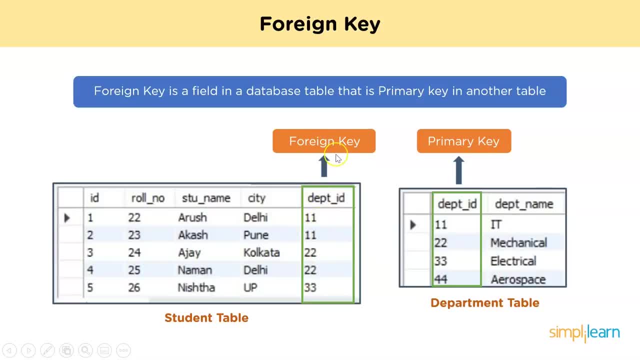 In the student table the department ID is the foreign key, whereas in the department table the department ID is the primary key. So this means that the department ID column in the student table is referring to the primary key. department ID column in the department table. 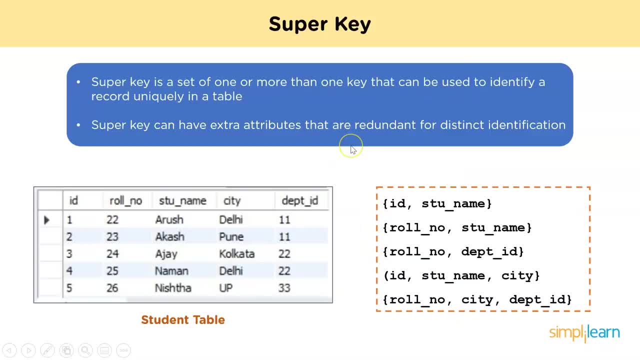 All right, so moving ahead, we have super key. This is a set of one or more than one key that can be used to identify a record uniquely in a table. So super key can have extra attributes that are redundant for distinct identification. So here we have the student table and on the right side you can see we have the list of. 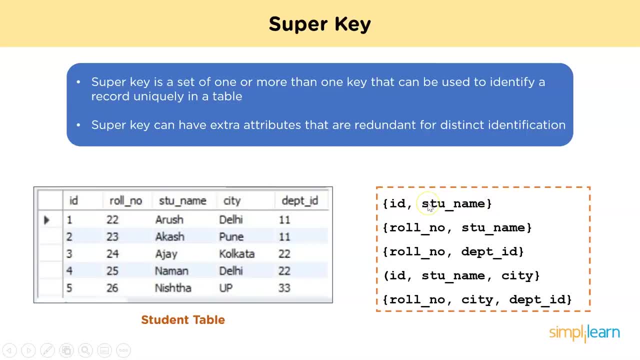 super keys. So using these columns you can identify each record in a table. So your ID and student name can be a super key. Similarly, role number and student name can be a super key. Then we have ID, student name and city combinedly, forming the super key. 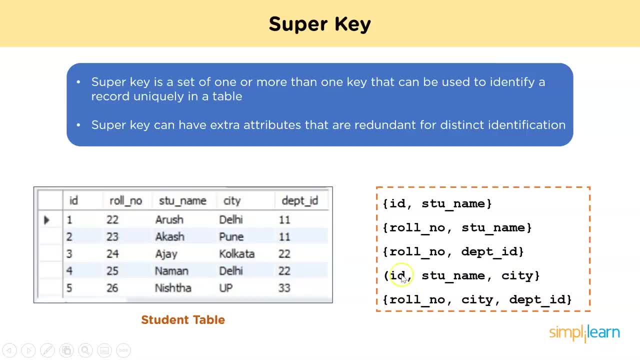 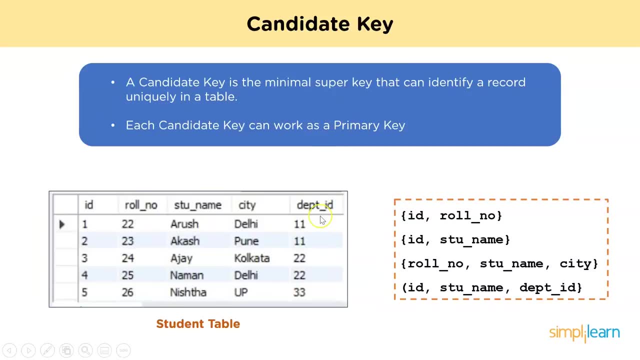 Then you also have the role number, city and department ID as a super key. There can be other combinations as well. Now moving to learning what is a candidate key. So candidate key is the minimal super key that can identify a record uniquely in a table. Each candidate key can work as a primary key. 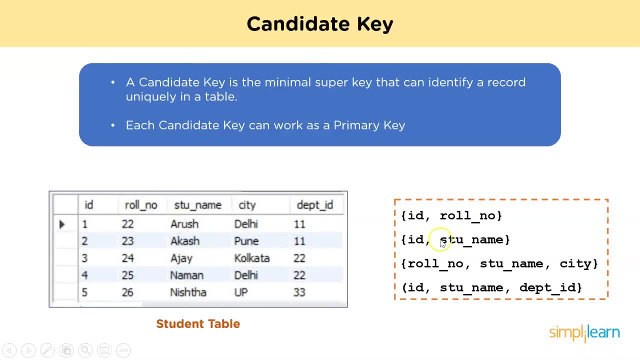 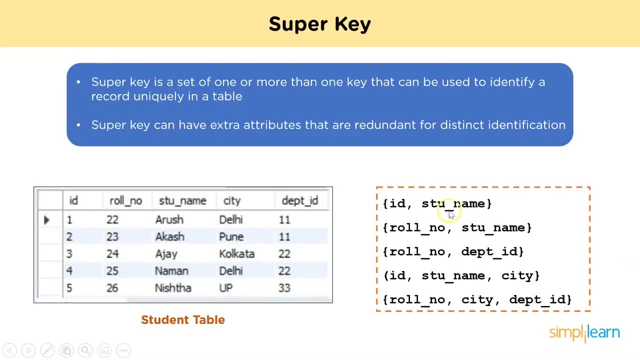 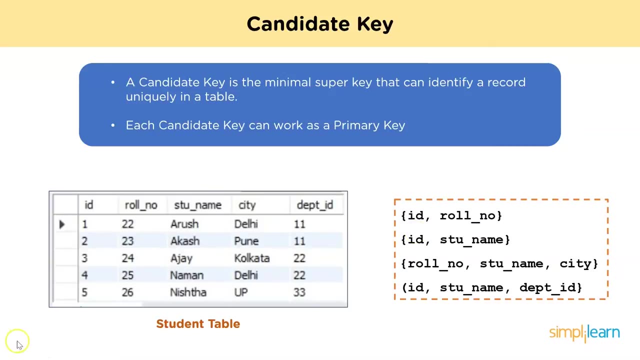 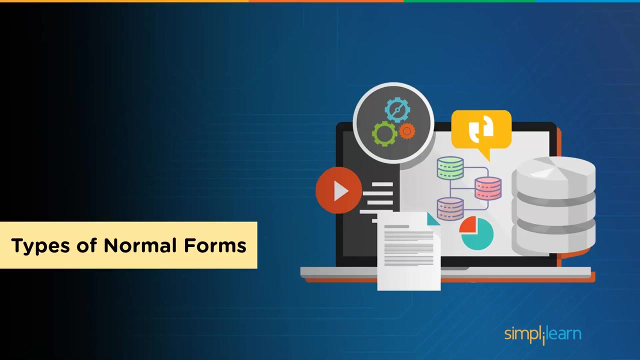 So we have the same table again And these are the list of candidate keys, just to make sure these candidate keys should be also part of the super key. So hence, a candidate key is also known as a minimal super key. Now, with this basic knowledge about the different keys in a database, let's look at the next topic. 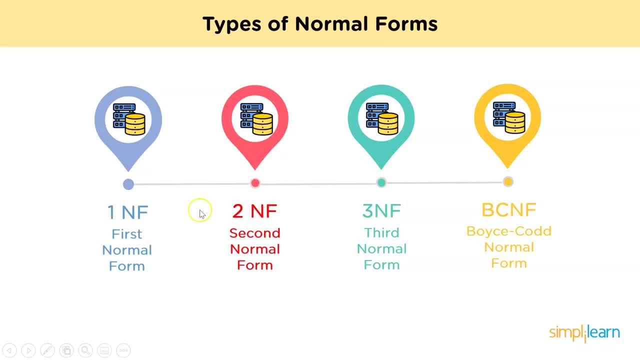 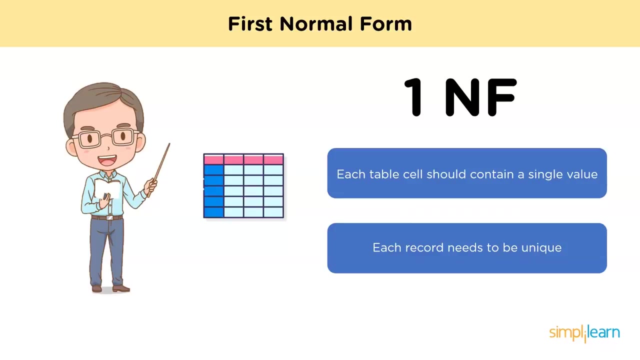 We have types of normal forms. So we have the first normal form, the second normal form, third normal form And BCNF or Boyce-Codd normal form that we are going to discuss in this session, Coming to learning what is first normal form. So a relation is in first normal form if it. 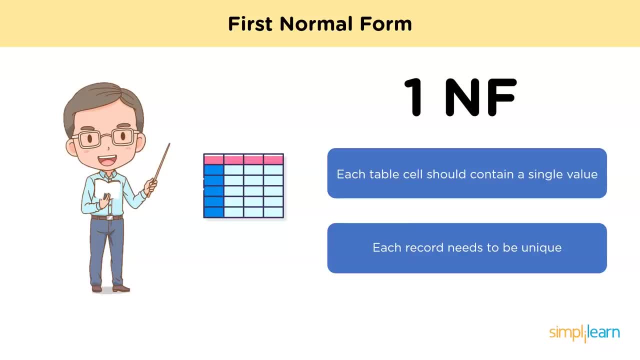 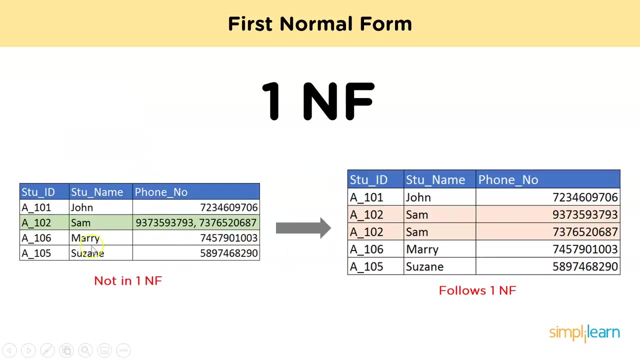 does not contain any composite or multi-valued attribute. So each table cell should contain a single value and each record needs to be unique. That is, an attribute of a table cannot hold multiple values. Let's see an example. So here you can see we have a student table and this table is not in first normal form because we 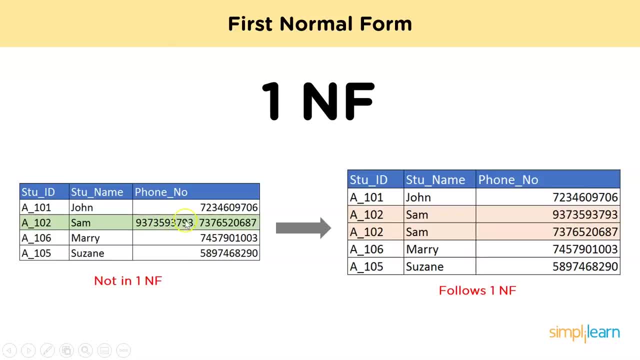 have multi-valued attribute: student phone number for student ID A102 with the student name Sam. So here we can see there are two phone numbers, So this becomes a multi-valued attribute. Now the table can be transformed to the first normal form like this You can see: 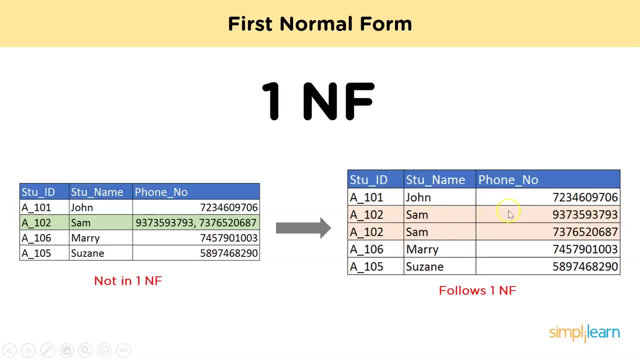 On the right side. So this contains only atomic values or single value in each cell. So we have split A102- Sam having two different phone numbers- into two different rows. Now this table follows the first normal form, because each of the cells have atomic values. All right, Now let's. 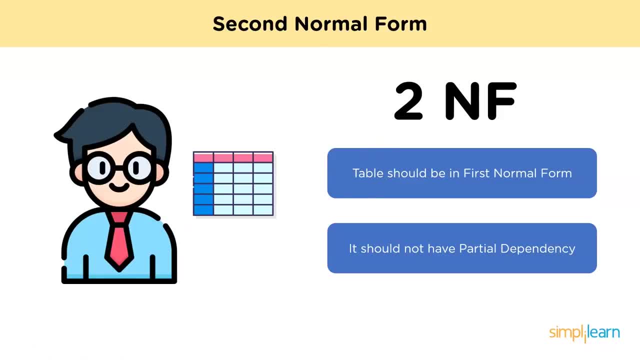 understand what is the second normal form in a database. So for a table to be in second normal form, the following two conditions should be met: The first is that the table should be in first normal form and it should not have any partial dependency, So records should not depend on. 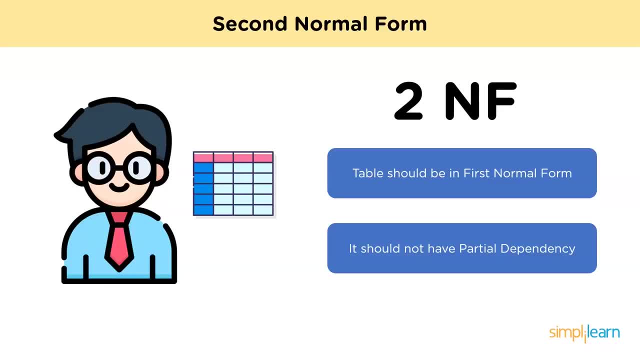 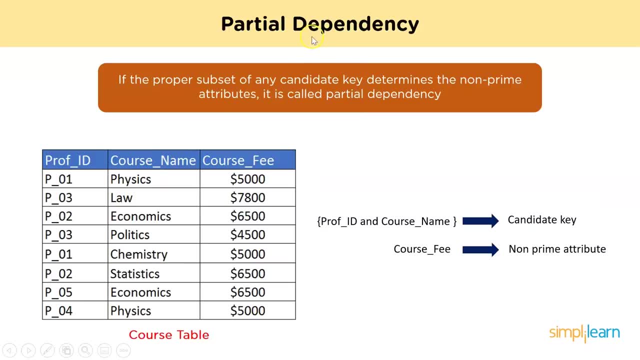 anything other than a table's primary key. Hence you need to remove subsets of data that apply to multiple rows of a table and place them in separate tables. Let's understand what is a partial dependency. So if the proper subset of any candidate key determines the 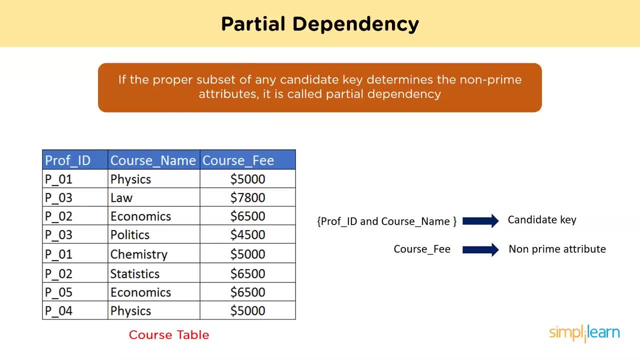 non-prime attributes. it is called partial dependency. Let's understand this with an example. So here we have a course table and the table has three columns. We have the professor ID, then we have the course name and then we have the course fee. Now the course fee attribute. 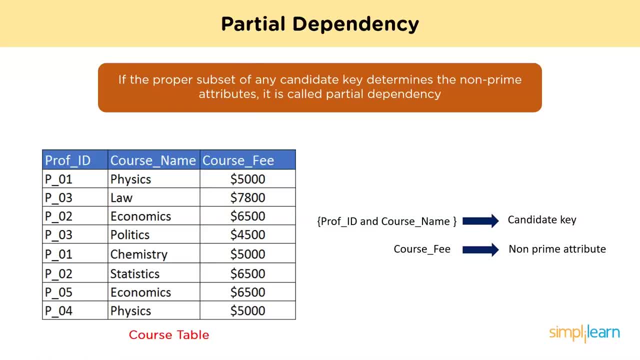 cannot alone decide the value of professor ID or the course name. Similarly, the course fee to be together with professor ID column cannot decide the value of the course name. Course fee column together with the course name column cannot decide the value of professor ID, Hence course fee column. 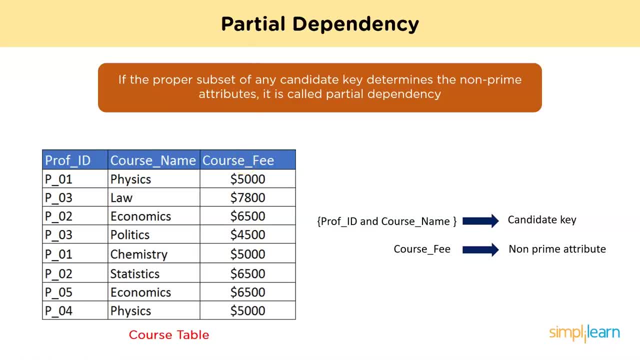 here becomes the non-prime attribute as it does not belong to any of the candidate keys, that is, the professor ID and the course name. But here the course fee column is dependent on the course name. Course fee of a particular course. you need to know the course name. 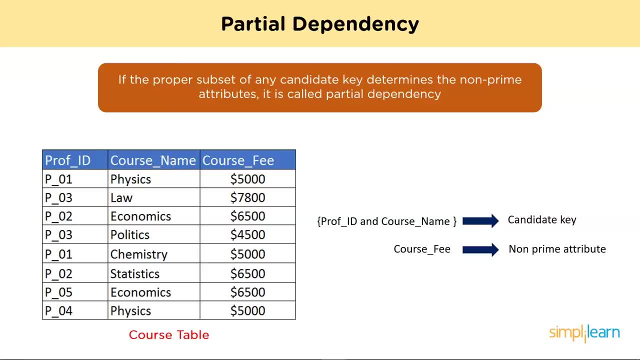 Course name column. here is a proper subset of the candidate key. So the non-prime attribute, which is the course fee, is dependent on a proper subset of the candidate key. Now this creates a partial dependency, So this relation is not in 2NF. Here you can see we have the professor ID and course. 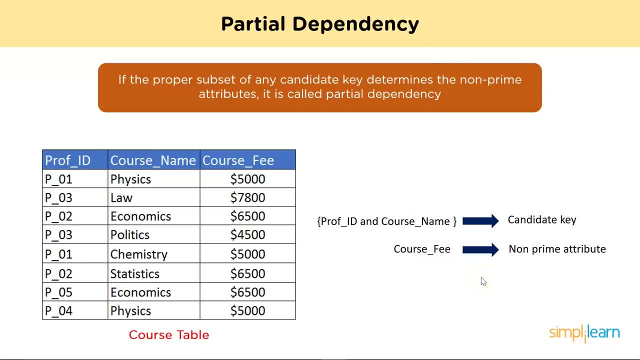 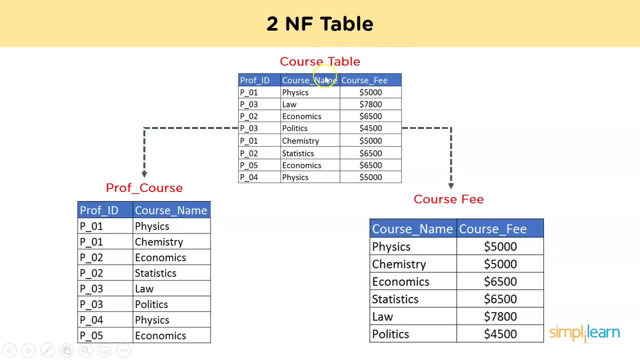 name combinedly forming the candidate key and course fee is the non-prime attribute. Now to convert this table into second, normal form, we need to split the table into two tables. Here you can see we have our original course table and we have split into two tables. That is the 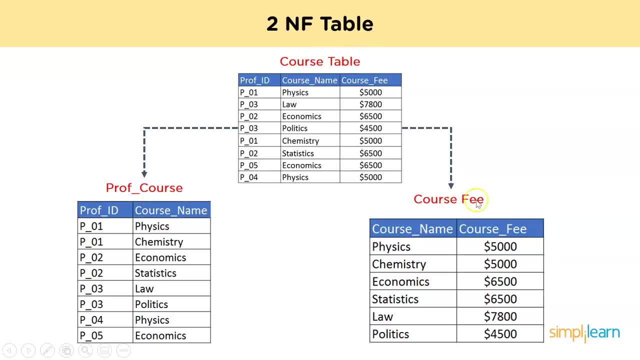 professor course table and the course fee table. So the professor course table has two columns: the professor ID and the course name. Similarly, for course fee have the course name. So these are all unique courses. Now here we can see we have the course fee table and we also have the course fees for the course. 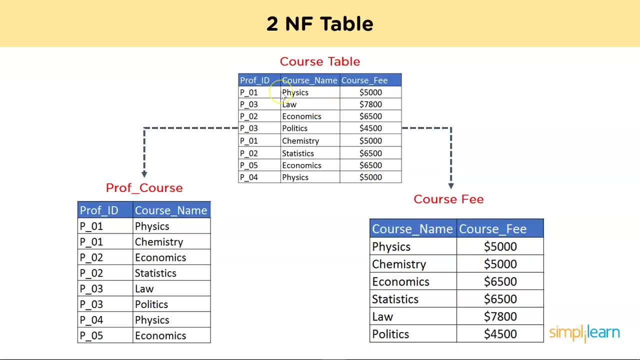 fee. Now, one thing to notice here is a lot of the courses are been taught by the same professors. For example, professor ID P01 teaches both physics and chemistry. Similarly, professor P03 teaches law and politics, and professor P02 teaches economics and statistics. 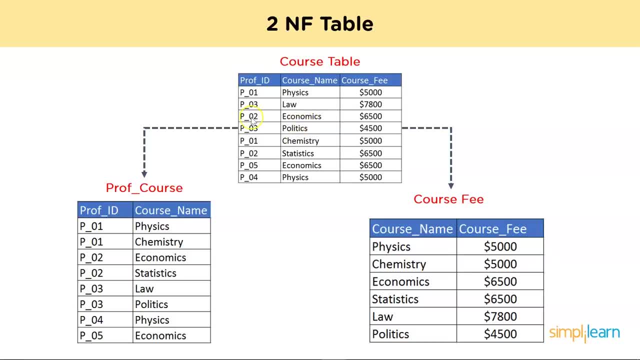 multiple professors for each of the courses. for example, for economics, we have p02 and p05. for physics, we have p01 and p04 as well, and the course fees for a few of the courses are the same. for example, for physics and chemistry, the course fee is five thousand dollars. similarly, 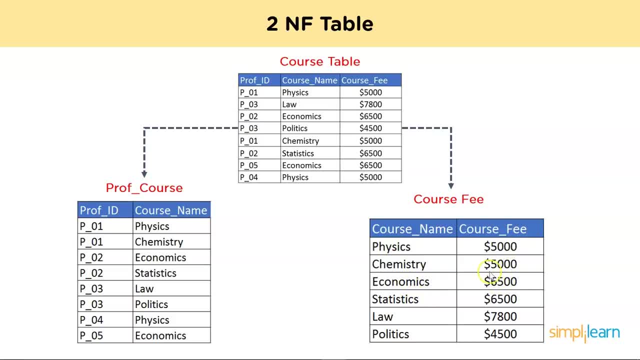 for economics and statistics. the course fee are the same, so six thousand five hundred dollars now. the second normal form tries to decrease the unnecessary data getting stored in memory. for example, if there are 10 professors teaching the chemistry course, we don't need to store its fee as 5000 for all the 10 records. instead, just once we can store it in another table as the 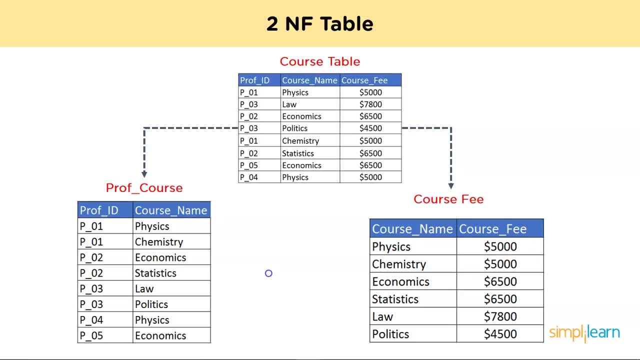 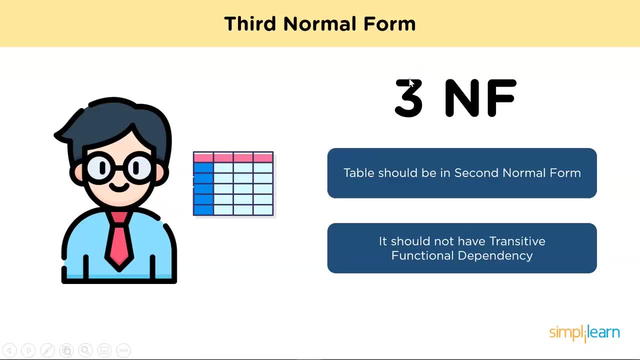 course fee for chemistry is five thousand dollars. now let's move on to the next normal form. we have the third normal form. now let's move on to the next normal form. we have the third normal form. so a relation is said to be in 3nf for third normal form if it is in second normal form and 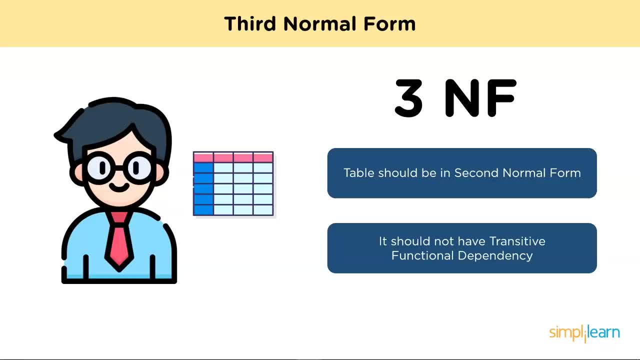 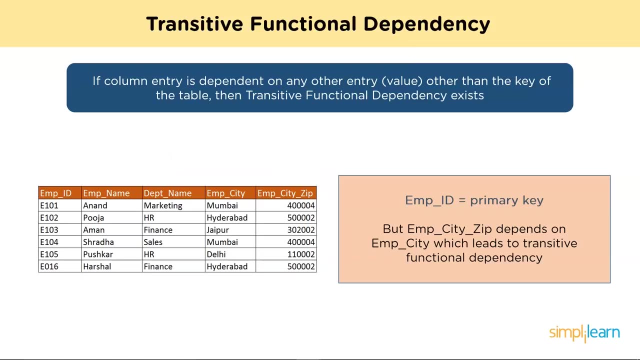 does not contain any transitive partial dependency. the 3nf is also used to diminish data duplication and it is also used to achieve data integrity. let's understand what is transitive functional dependency with an example. so a transitive functional dependency exists if the column is: 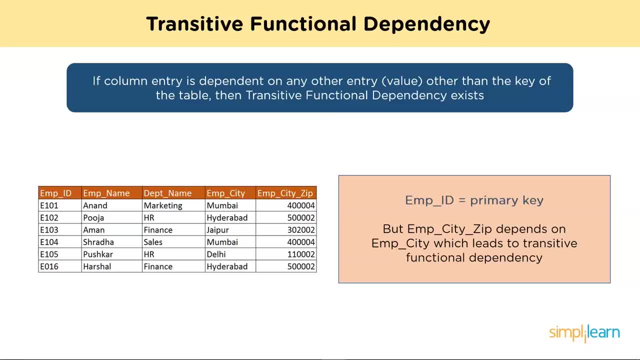 entry is dependent on any other column apart from the key column in the table. so here we have an employee table and in this table we have the employee ID as the primary key. also, the candidate key in this table is the employee ID and there are a few functional dependencies. for example, the employee name is 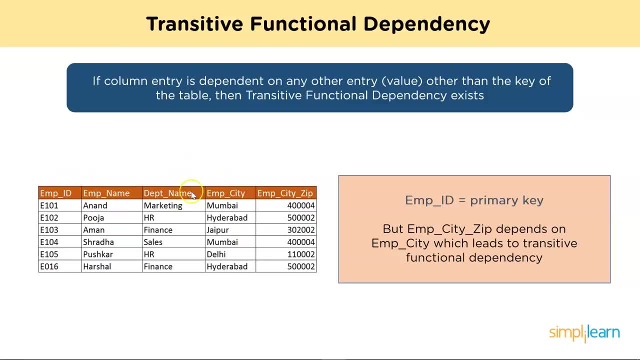 dependent on the employee ID. similarly, the department name of the employee is dependent on the employee ID column. we have the employee city depending on the employee ID column again, but the city zip code or the city pin code is dependent on the employees city name, for example, if you want to know the zip code. 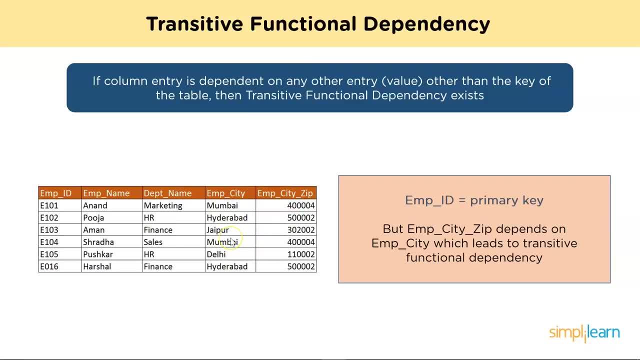 of a particular place, you need to know the name of the place or the city. so hence your employee city zip column depends on the city column and this leads to a transitive functional dependency. so we need to break the table into two tables for transforming it into the third, normal form. now let me show you how you. 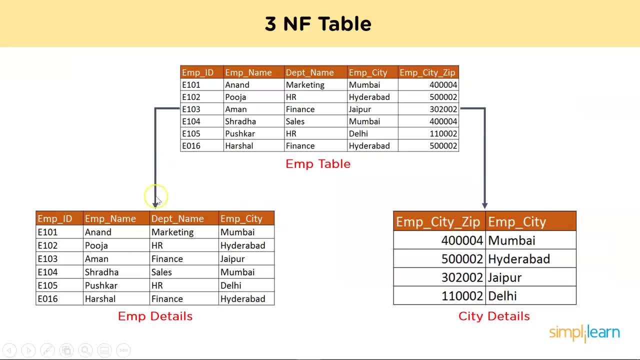 can break it in the next slide. so here you can see, we have the original employee table with all the columns. and now we have broken our original table into two columns. so here you can see we have the original employee table with all the columns. and now we have the original employee table with our command line. 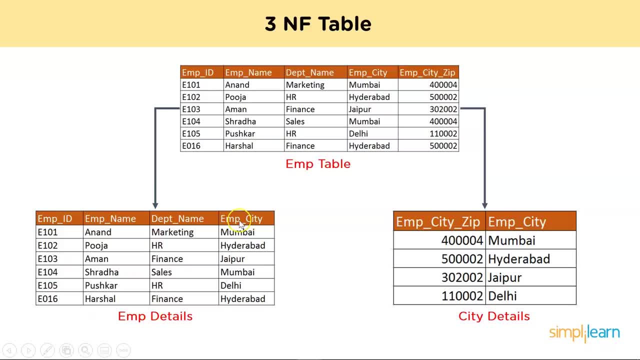 and here we have the condition of this name, employee details and city details. so here your employee ID becomes the primary key and we have the employee name, department name and the employee city. so each of the other non-prime attributes are depending only on the primary key or the candidate key here. 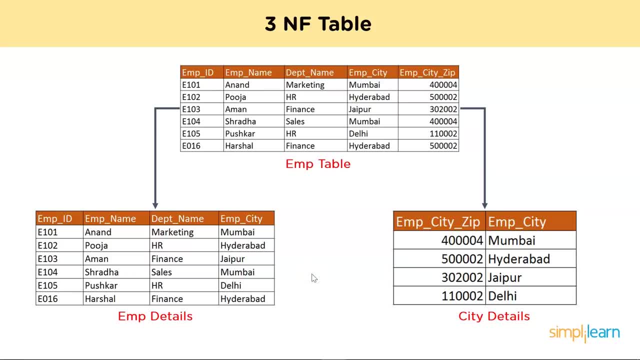 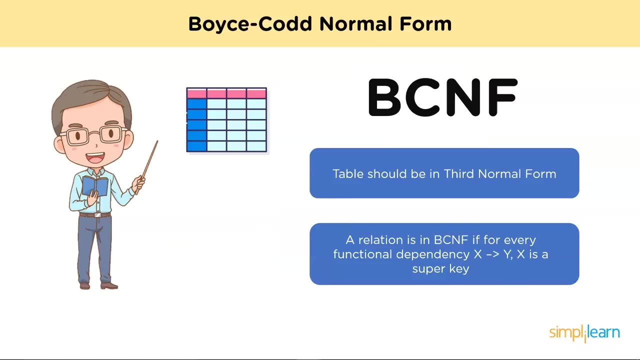 city for each of the zip codes. all right, so this tells us that all the non-key columns are fully functional, dependent only on the primary key column. now moving ahead to the next normal form, which is the boy scott's normal form. so boy scott normal form, or bcnf, is a special case of third. 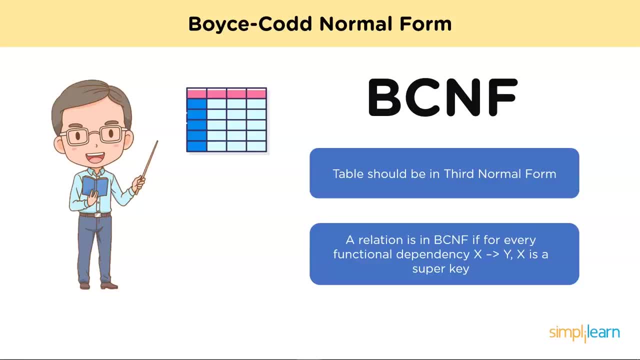 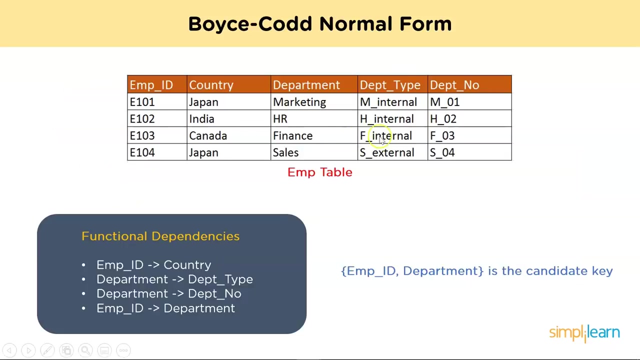 normal form a relation is in bcnf if, and only if, every determinant is a candidate key. so if for every functional dependency x determines y, here x should always be a super key- only then the relationship is in bcnf. now let's see an example. so here we have an employee table with the columns: 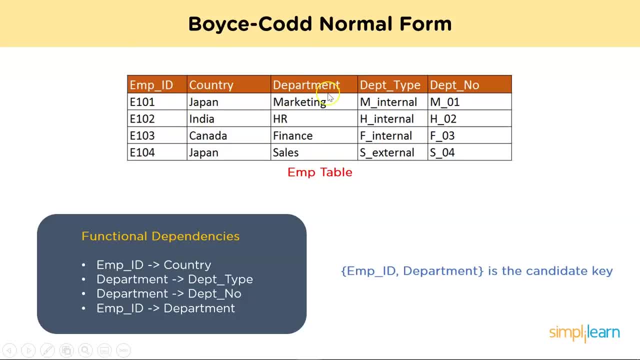 employee id, the country to which the employee belongs to. you have the different departments. we have the department type and the department number as well. so here one thing to note. you can see there are two employees from japan, that is, from the same country, but these are two different employees. now you can see the functional dependencies that 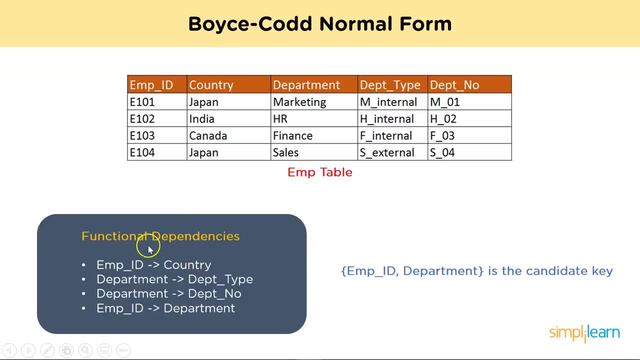 exist. so to know the country of the employee you need to know the employee id. so your country is dependent on employee id. similarly, your department type- column- is dependent on the department column. department number is also dependent on the department column. and to know the department you need to know the employee id. so here your employee id. and. 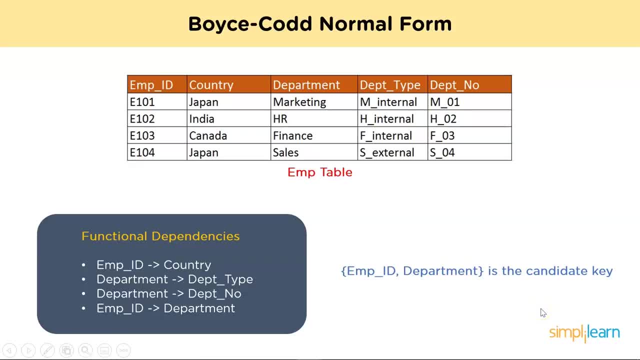 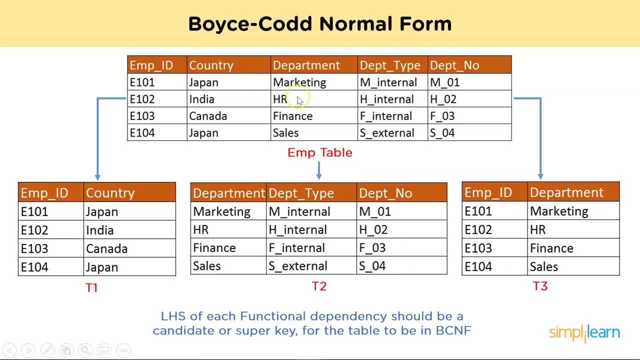 department columns together form the candidate key. now to transform the above table to boy scott normal form of bcnf, we have to break it down into three tables. you can see here t1, t2 and t3. so in the first table we have employee id as the candidate key or the super key, and then 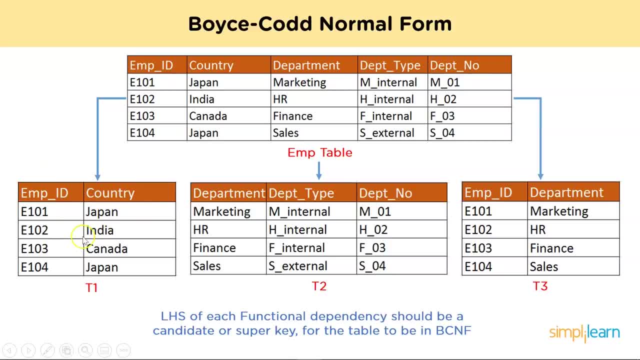 we have the country, so your country is dependent on the employee id. similarly, in table t2, your department type column and department number columns are dependent only on the department column and in the third table, that is, t3, your department is dependent on the employee's id. 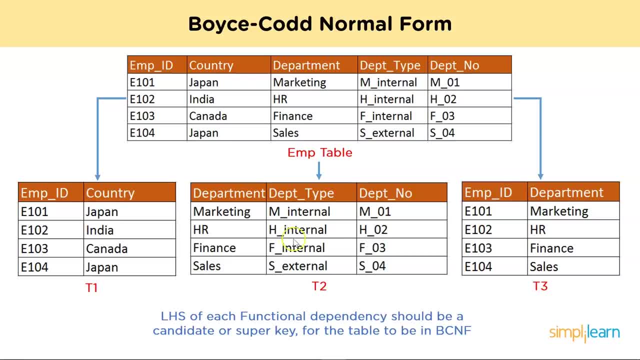 so here the candidate keys for tables t1, t2 and t3 are employee id department and employee id and department together. so one thing to notice: the lhs or the left hand side of each functional dependency should be a candidate or super key for the table to be in bcnf. and that brings us to the end of this. 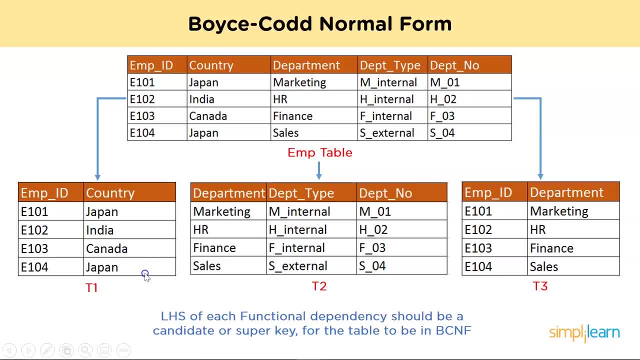 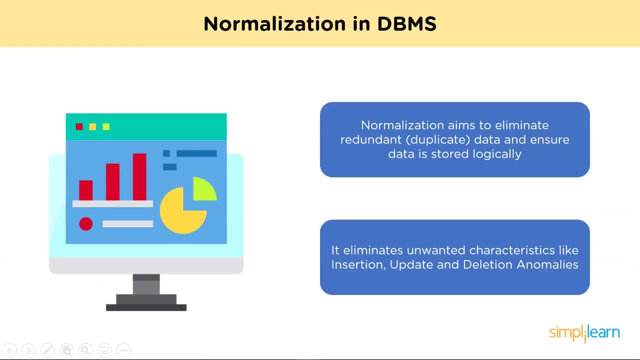 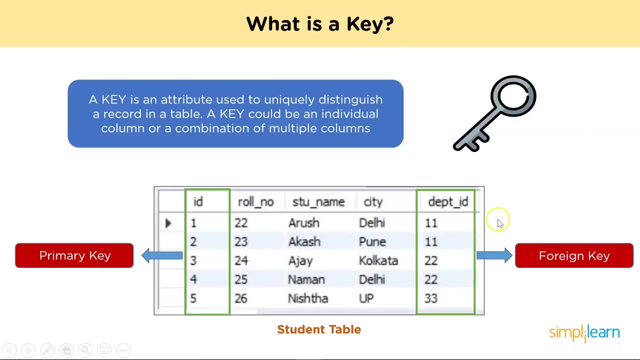 video tutorial on normalization in bcnf dbms. let me just run through whatever we learned. so first we looked at the basics of normalization in database management system and why do we need it. then we learned what is a key in a database table. then we looked at the different types. 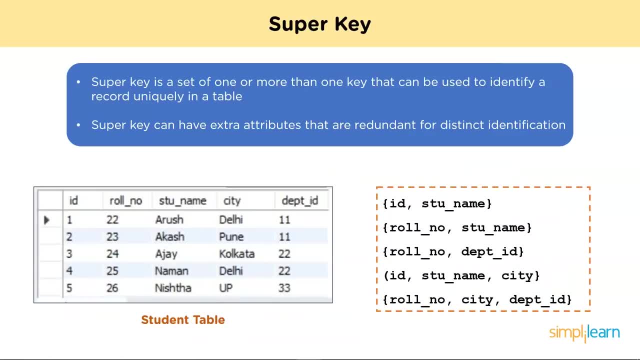 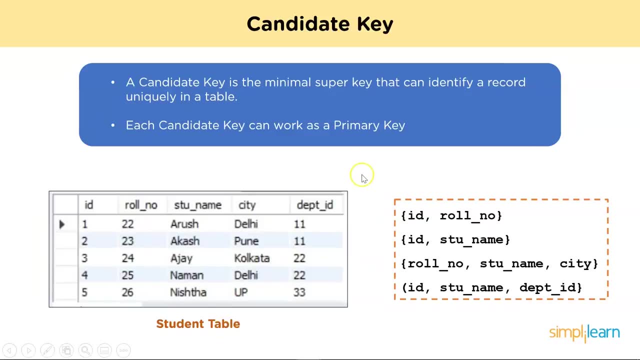 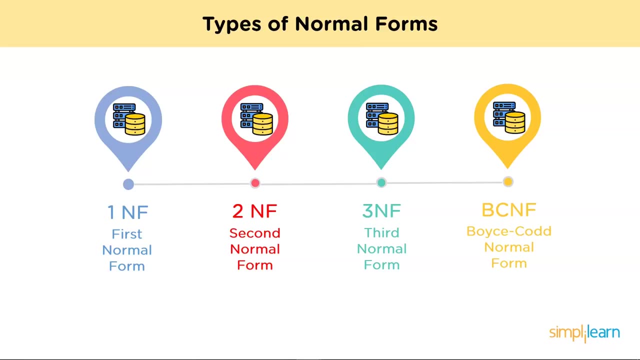 of keys. so we understood what is a primary key, what is a foreign key. then we looked at what is a super key and we listed down a few super keys for our student table. then we understood how candidate key is related to super key and then we moved ahead with our types of normal forms. so we 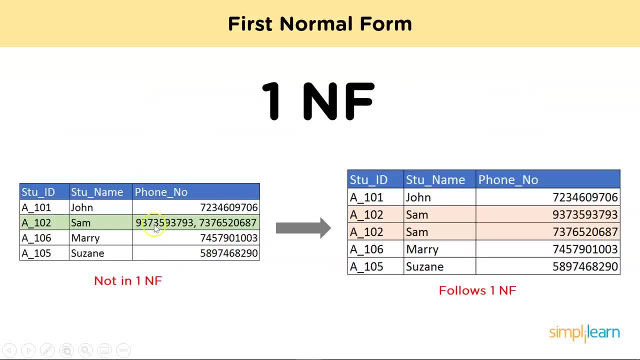 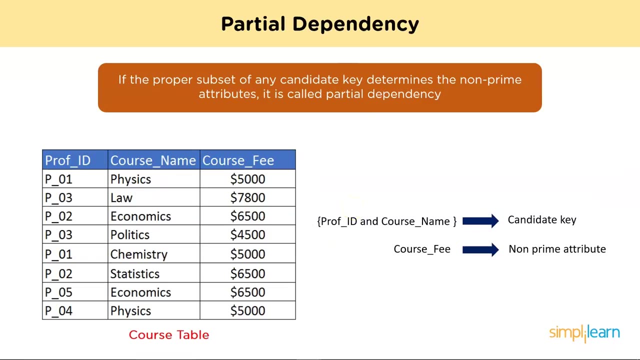 explored the first normal form. so we learned here that all the values in the table should be atomic. so we broke our rows into two different rows for the table to be in first normal form. then we understood about the partial dependency in a second normal form and how you can avoid partial 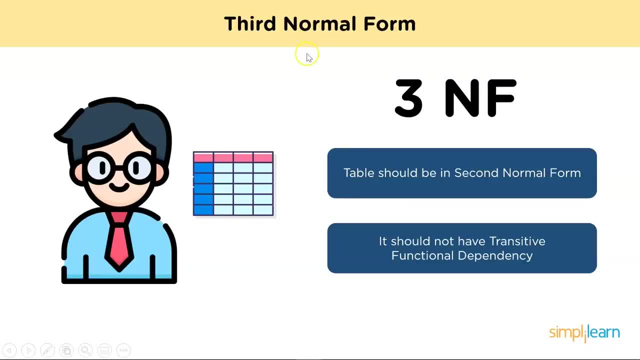 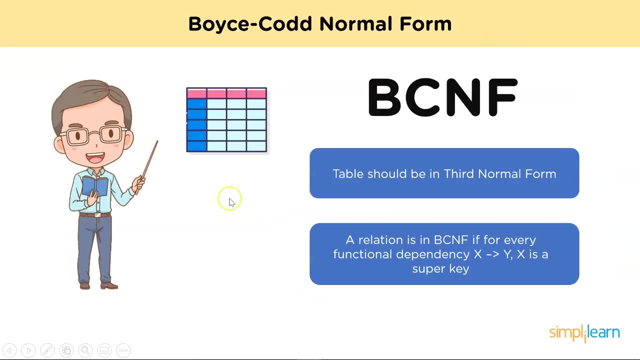 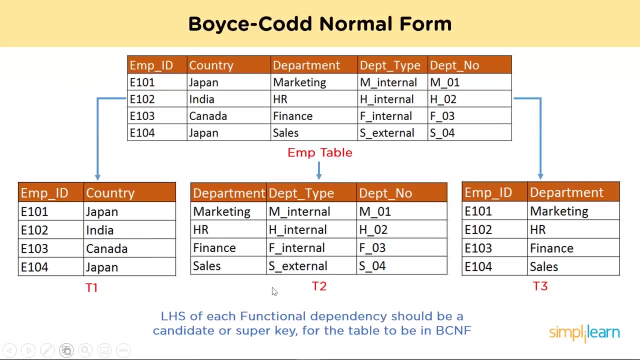 dependency in a table. then we looked at the third normal form and understood about the transitive functional dependency using this employee table and finally we learnt about the boy squad normal form with an example. now there are other normal forms as well, such as the fourth normal form and the fifth normal form, but in most of the cases, in reality, all the 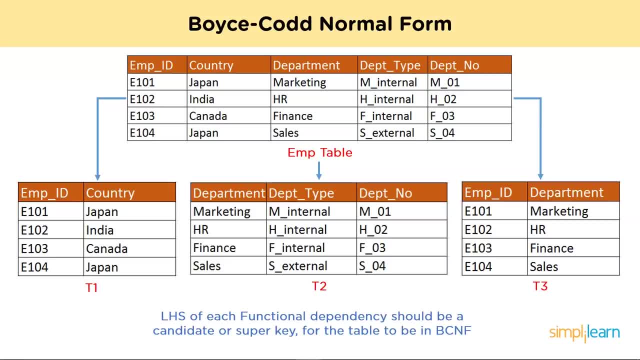 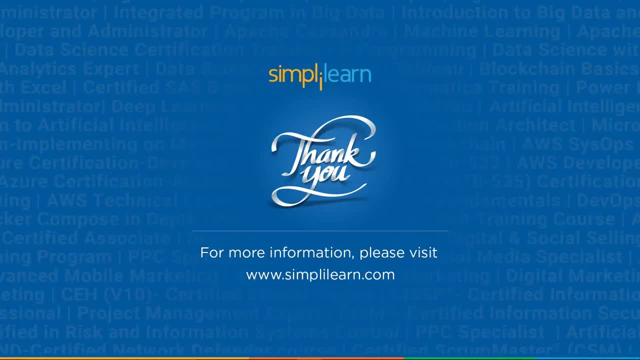 data integrity issues and the anomalies such as the insertion, deletion or update anomalies, are resolved in the third normal form or the BCNF form. Cool, Thank you all for watching this video tutorial on normalization in DBMS. I hope this was useful and interesting. If you have any queries, 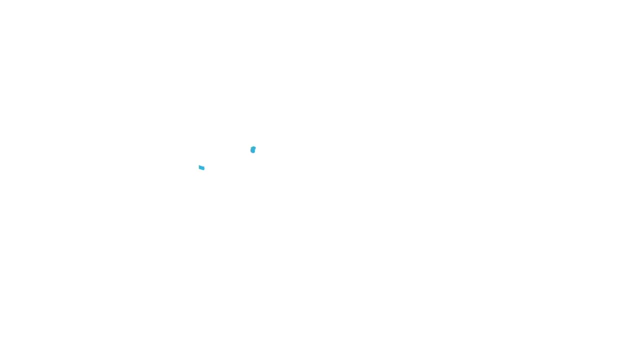 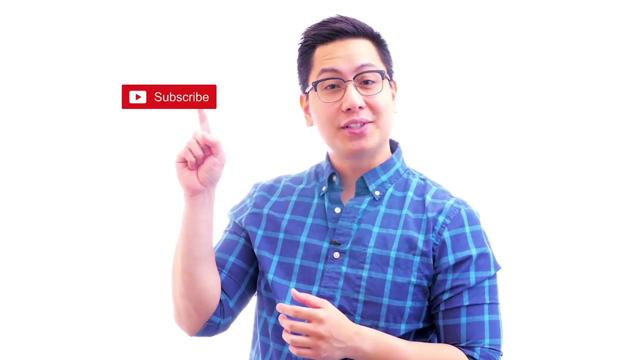 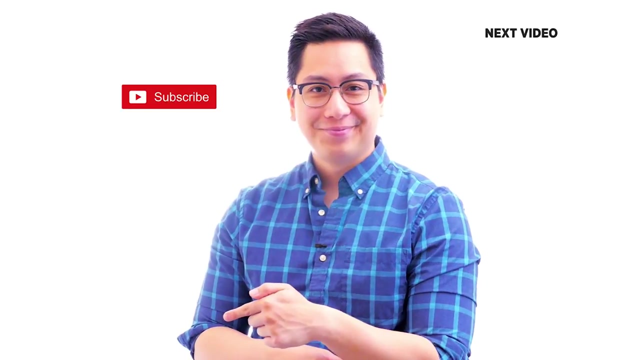 please feel free to put them in the comment section below. Thanks for watching. Bye.